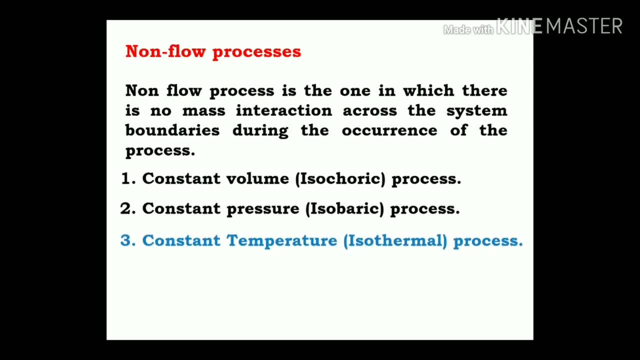 process, or you can say the isobaric process, Constant temperature process, or you can say the isothermal process. So today we will only focusing on to the constant temperature process or isothermal process. Then one more adiabatic process in which there is no heat transfer. Five number the: 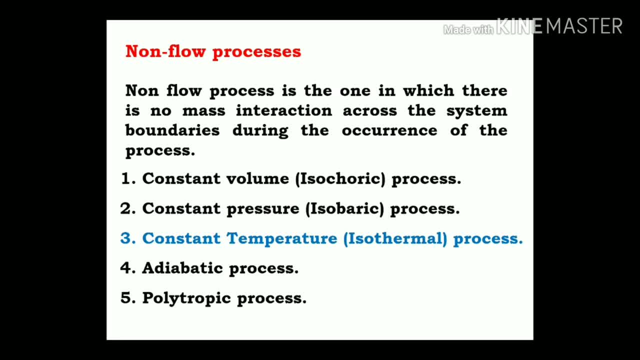 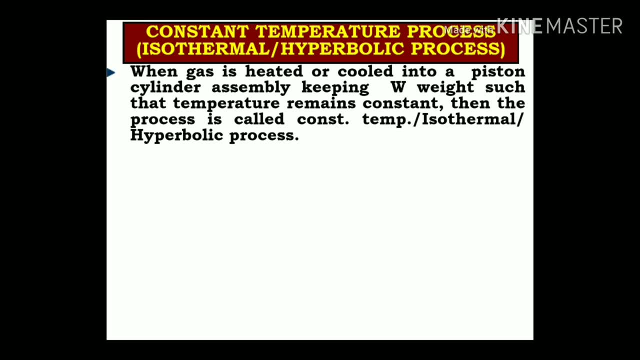 polytropic processes. So let us start the constant temperature process, or you can say the isothermal or hyperbolic process. So generally in the constant thermal process, when a gas is heated or cooled in a piston cylinder assembly keeping W weight such that the temperature remains constant, then the process is called as a. 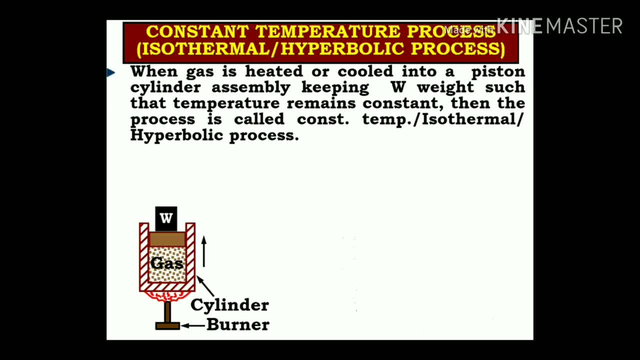 constant temperature or isothermal, or hyperbolic process. So let us say on to the P-V diagram: x-axis representing the volume and y-axis representing as a pressure. So in which state number one, or point number one, P1, V1, and just, it will be changing from one state to another. 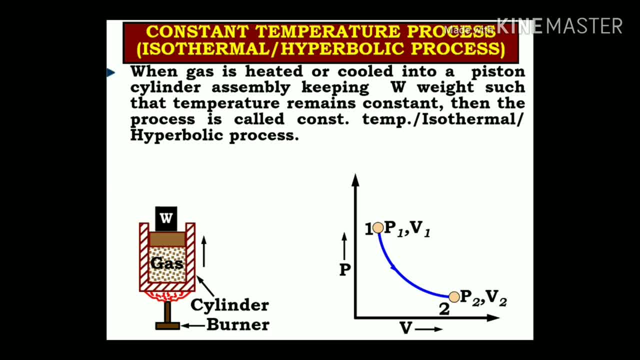 state at constant temperature. So that will be P2, V2 at point number two. So that will be equal to P-V, equal to constants, and it will be nothing, but it will be said to be a boil. So in the case of boil, slow, T1 equal to T2, that means constant temperature process. In that case, 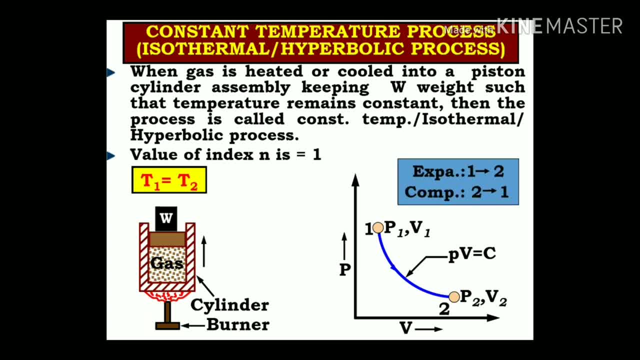 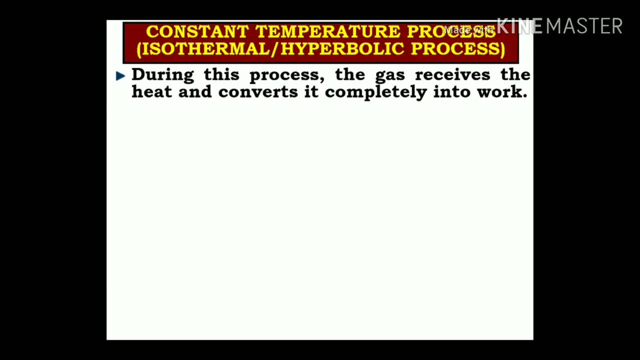 value of the index that will be equal to one. So during this process the gas receives the heat and converts completely into the works. So during this process, temperature remains constant and hence the change in internal temperature. So in this case the temperature remains constant and hence the 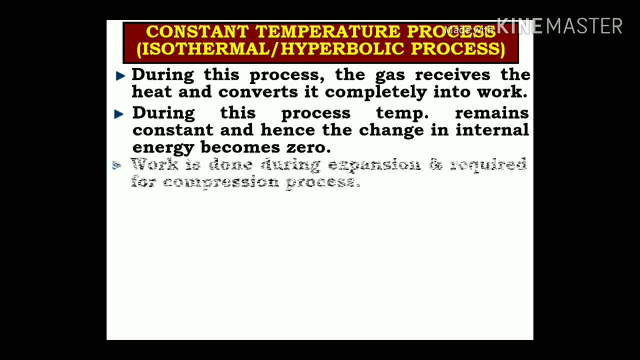 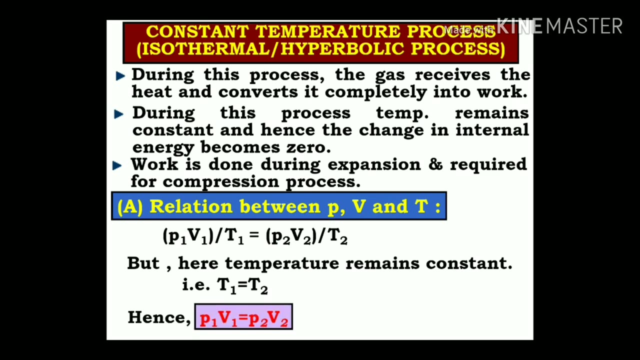 energy becomes zero. So work is done during expansion and required for the compression process. So relation between P-V and T, P1 V1 upon T1 equal to P2, V2 upon T2. in that case of constant temperature, T1 equal to T2. that means P-V equal to P1, V1 equal to P2 V2.. 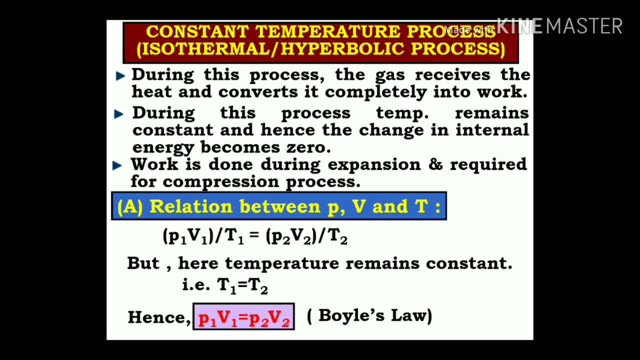 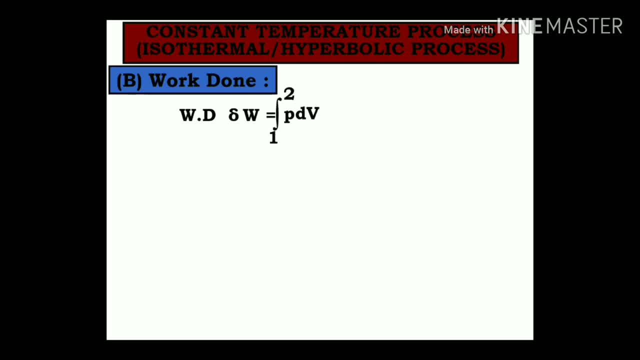 And that will be nothing but representing, as a boil, slow. So work done. in the case of constant temperature, process 1 to 2, process P into D, V, But P1, V1 equal to P, V equal to constant, So P equal to constant upon V. 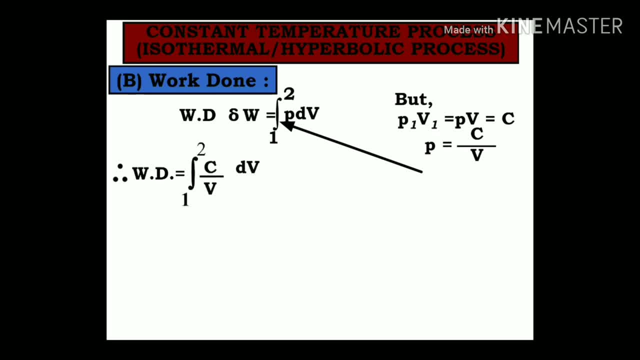 So let's put the value of the P into equations. So for 1 to 2, process C by V into D, V, then C into 1 to 2, process 1 by V into dV. so P1, V1, 1 to 2 process 1 by V, that will be. 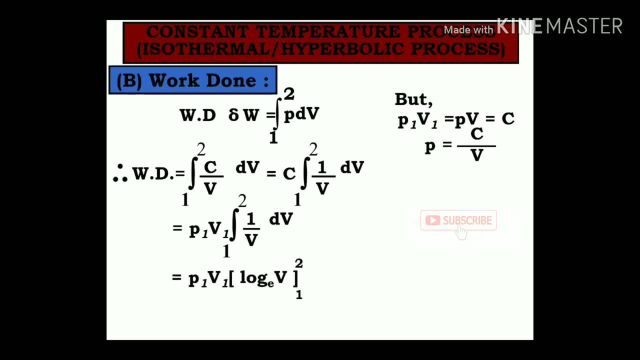 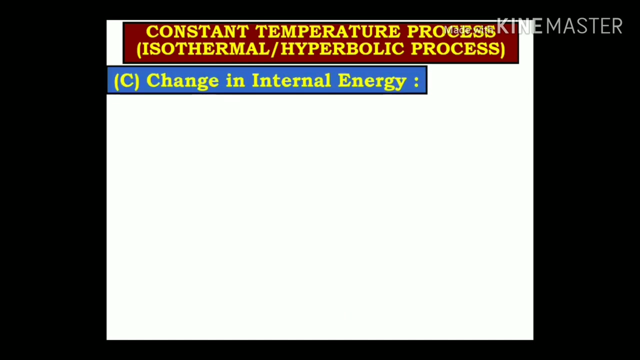 into dV. so P1- V1. finally log of E, V1 to 2 process. so finally work done: P1- V1, log E, V2 by V1, that will be representing over here at for the constant temperature process. so V2 by V1 equal to P1 by P2, so at constant temperature change in internal energy that will. 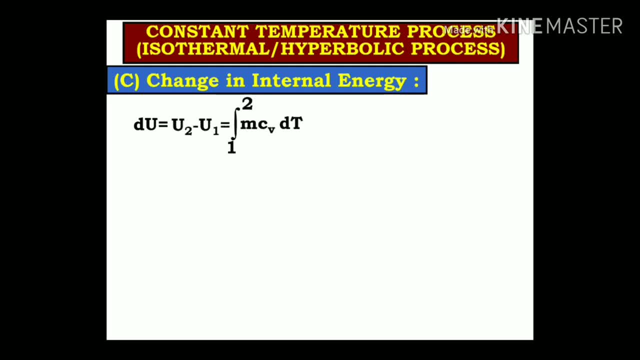 be du equal to u2 minus u1 and that will be equal to 1 to 2 process mcv delta t. so du that will be equal to mcv delta t. mcv t2 minus t1 kilojoule. but for isothermal process, t1 equal to t2, that means du equal to 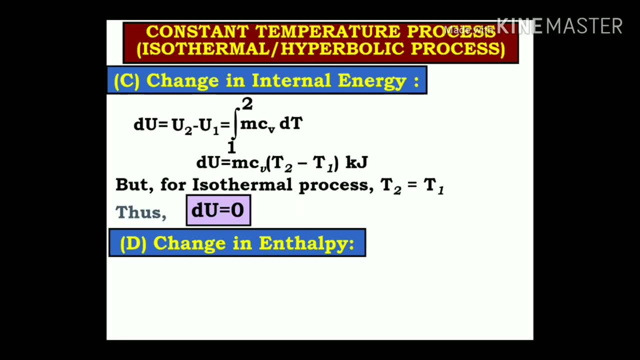 zero, so there is no internal energy store into systems. now we were discussing with the change into enthalpy, so dh equal to mcp. t2 minus t1, that will be the similar isothermal process. t2 equal to t1, so dh equal to zero. so that means change in enthalpy of the system at constant temperature. 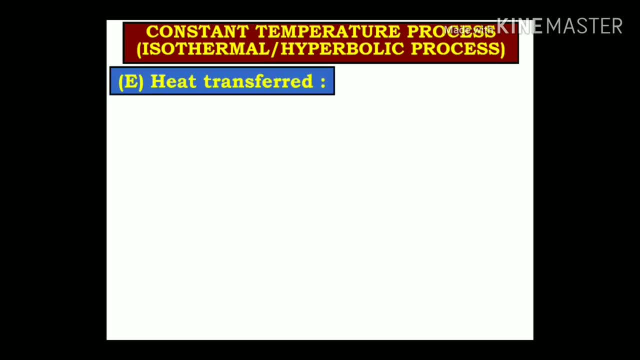 it will be zero. next, heat transfer. so as for the first law of the thermodynamics, del q equal to del w plus du, that means heat supplied equal to work done plus store energy. so here du equal to zero because at constant temperature process. so dq equal to dw, that means what heat supplied on the systems. it will be 100% converting.